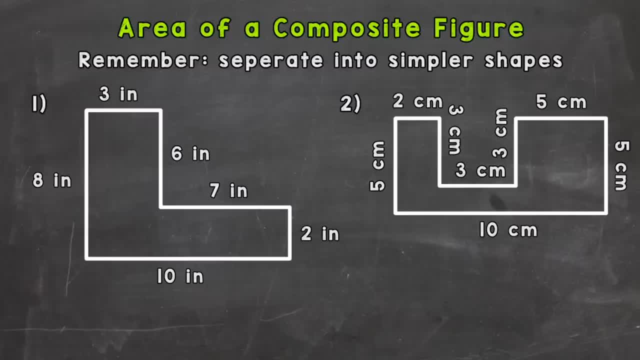 the first thing I want to do is again separate into simpler shapes. So I'm going to cut this into two rectangles. I'm going to draw a dashed line here to represent where I'm cutting it Now. I'm going to name the left rectangle A and the right rectangle B And it's going to. that's going to help keep me. 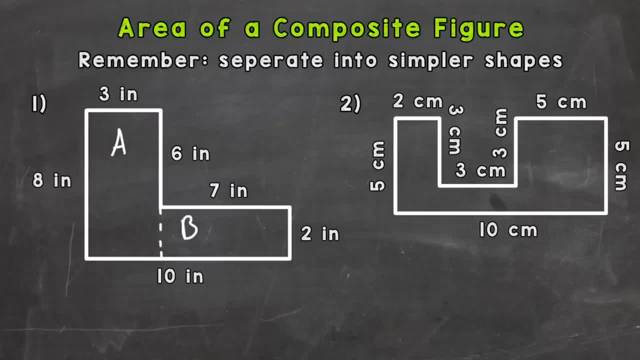 organized as I work through this problem. So I know that finding the area of a rectangle area equals length times width. So now let's find the area of our rectangle A and rectangle B, So A and B, So area equals length times width. All right, now I need to plug in. 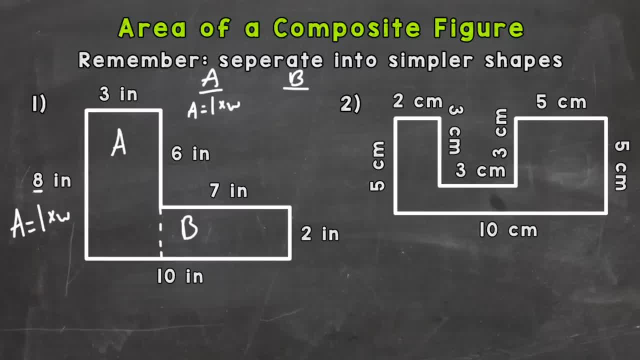 length and width. So my length for A is going to be this: 8, all the way up right. Don't use this 6, because this 6 doesn't go the full length of the rectangle, So you have to be careful which measurements you use. So I'm going to use this 6.. So I'm going to use this 6.. So I'm going to use. 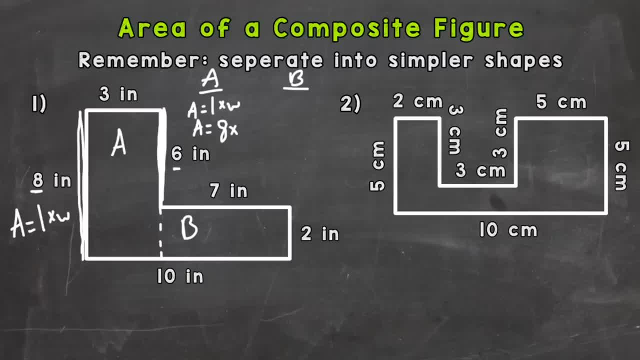 the 8. And I'm going to multiply it by the width of 3. And that gives me an area of 24 square inches. So the area of A area equals 24 square inches. Now let's do B Area equals length times. 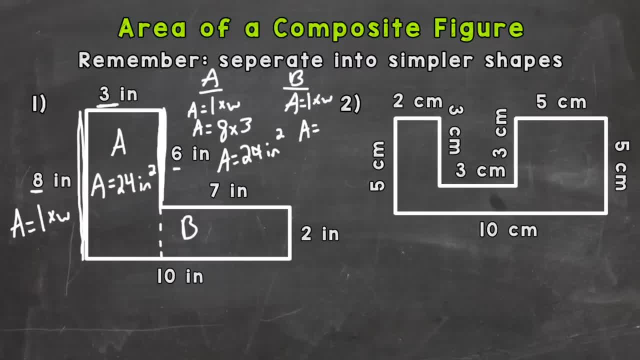 width, Let's plug in. Length is going to be this 2.5.. So I'm going to use this 2.5.. So I'm going to use the 8. And I'm going to multiply it by the width of 3. And that gives me an area of 24 square. 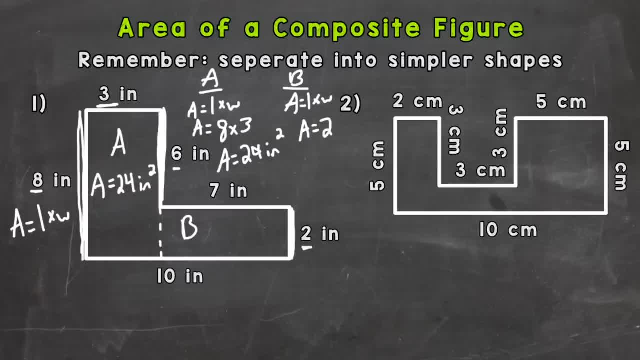 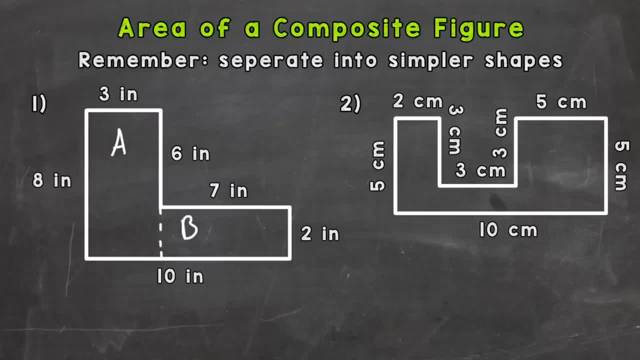 organized as I work through this problem. So I know that finding the area of a rectangle area equals length times width. So now let's find the area of our rectangle A and rectangle B, So A and B, So area equals length times width. All right, now I need to plug in. 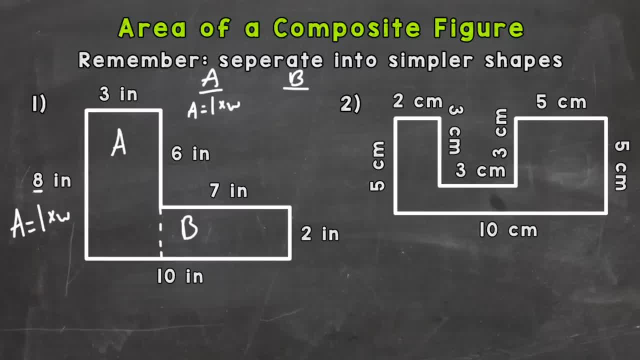 length and width. So my length for A is going to be this: 8, all the way up right. Don't use this 6, because this 6 doesn't go the full length of the rectangle, So you have to be careful which measurements you use. So I'm going to use this 6.. So I'm going to use this 6.. So I'm going to use. 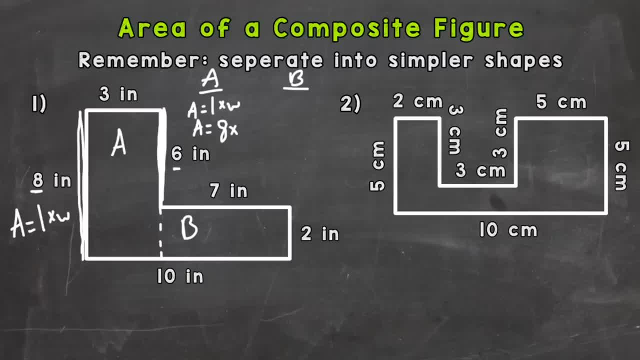 the 8. And I'm going to multiply it by the width of 3. And that gives me an area of 24 square inches. So the area of A area equals 24 square inches. Now let's do B Area equals length times. 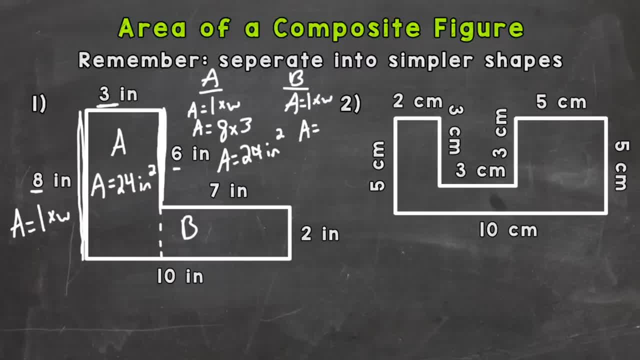 width, Let's plug in. Length is going to be this: 2, all the way up, right. Don't use this 6.. So I'm going to 2 inches here, So 2 times the width of 7 inches. Do not use the 10. The 10 goes all the way across. 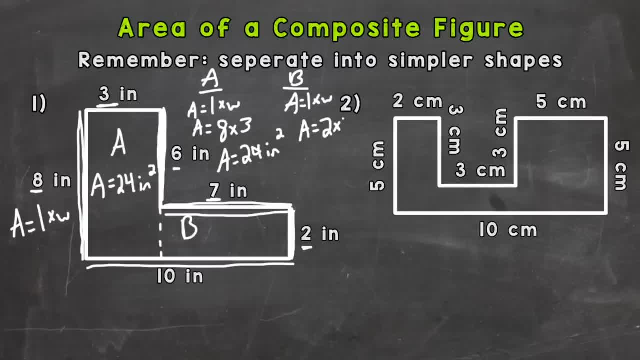 We only want right here, which is that 7 inches. So area equals 2 times 7, 14 square inches. So the area for B is 14 square inches. So now that we have the left rectangle and the right rectangle, the area of those, we add those together in order to get the area of the whole shape. So we would do 24 plus that 14. And that gives us an answer of 38.. 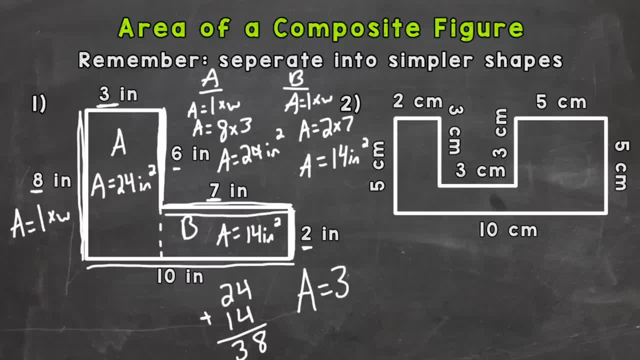 So our final area is 38 square inches. So again, we separated into simpler shapes and then found those areas, added them together for the area of the whole composite figure. Now for number one. we could have cut that this way as well and made a top and a bottom rectangle. 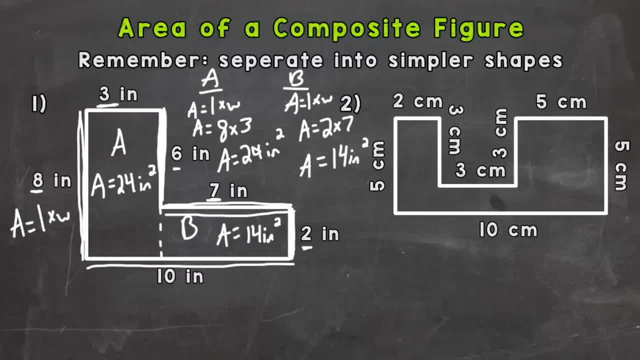 So now that we have the left rectangle and the right rectangle, the area of those, we add those together in order to get the area of the whole shape. So we would do 24 plus that 14. And that gives us an answer of 38.. 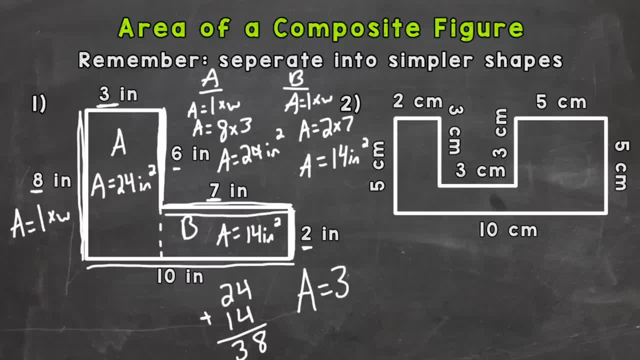 So our final area is 38 square inches. So again, we separated into simpler shapes and then found those areas, added them together for the area of the whole composite figure. Now for number one. we could have cut that this way as well and made a top and a bottom rectangle. 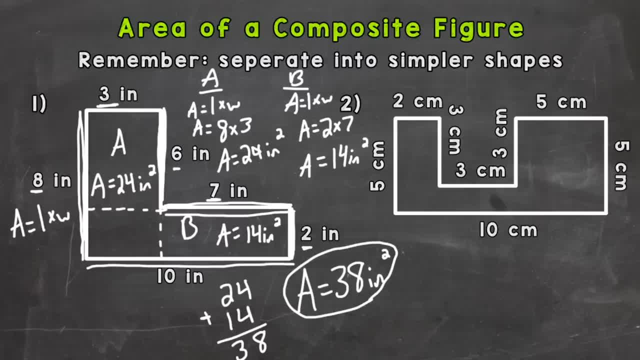 So usually there's multiple ways to separate a composite figure. It doesn't matter which way you separate it, but it does matter which numbers you use, which dimensions you use going around for your length and width. So that's something you need to be careful of. So let's jump into number two here and see how we do this one. This one's a little more complex. 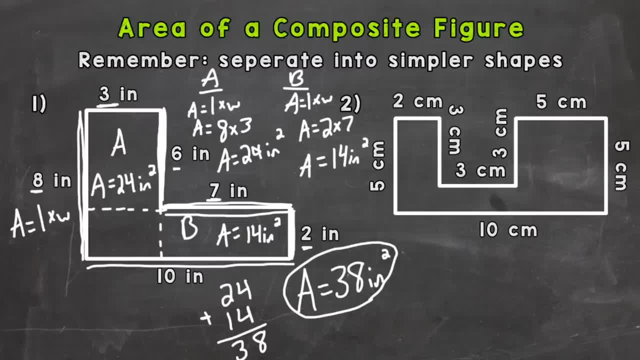 Now for this one. I'm going to cut it into or separate it into three. So I have three simpler shapes here and I have two rectangles and a square. So I'm going to name A, B and C. So let's find the area of these three. So area equals length times width. I'll put my formula first and then we will plug in. 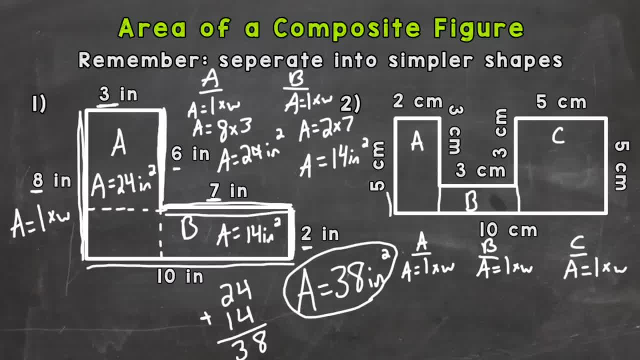 So for A, our length is going to be this. So our length is five all the way up. So we have five centimeters times the width of two centimeters, And that gives us an area of ten square centimeters. So let's do B. 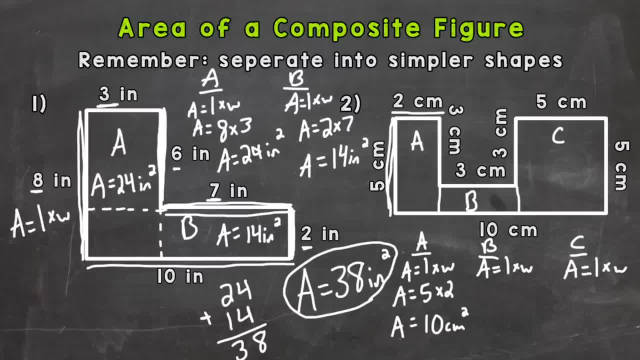 Now B, we have a length of right here or right here And we don't have a measure there, so we're going to need to figure it out. We know the whole shape is five centimeters, right? So if we have this three, what's this going to have to be in order to get us to that five centimeters? 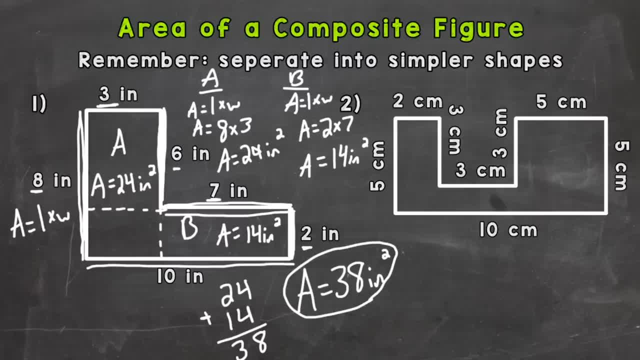 So usually there's multiple ways to separate a composite figure. It doesn't matter which way you separate it, but it does matter which numbers you use, which dimensions you use going around for your length and width. So that's something you need to be careful of. So let's jump into number two here and see how we do this one. This one's a little more complex. 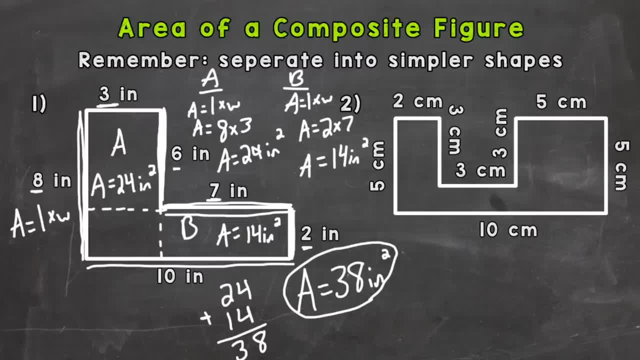 Now for this one. I'm going to cut it into or separate it into three. So I have three simpler shapes here and I have two rectangles and a square. So I'm going to name A, B and C. So let's find the area of these three. So area equals length times width. I'll put my formula first and then we will plug in. 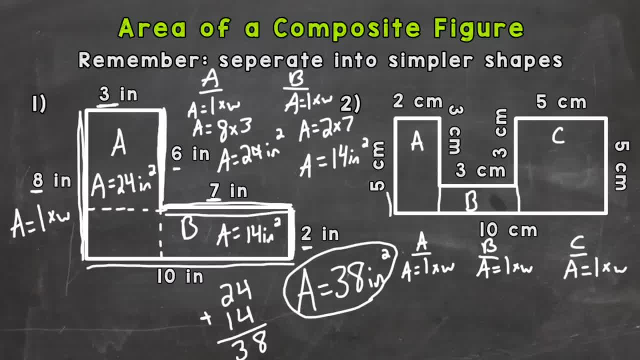 So for A, our length is going to be this. So our length is five all the way up. So we have five centimeters times the width of two centimeters, And that gives us an area of ten square centimeters. So let's do B. 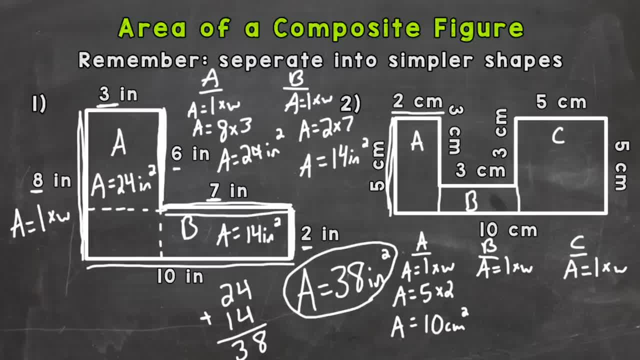 Now B: we have a length of right here or right here And we don't have a measure there, so we're going to need to figure it out. We know the whole shape is five centimeters, So if we have this three, what's this going to have to be in order to get us to that five centimeters? 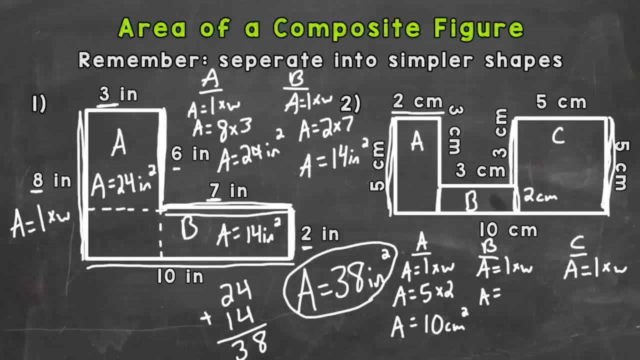 Well, it's going to have to be two centimeters, And again I figured that out because this three right here plus this two centimeters equals the total height of the five centimeters given to us on the left and right hand side. So sometimes in composite figures you have to figure out some measurements that aren't given. 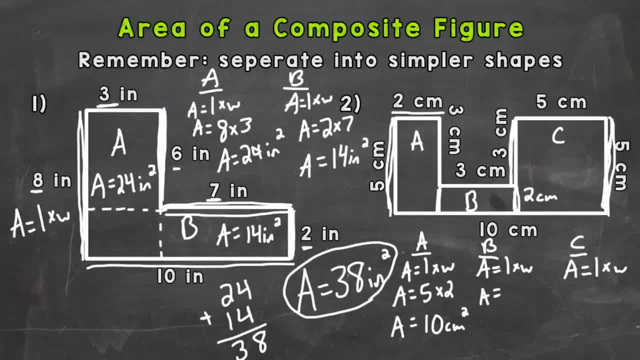 Well, it's going to have to be two centimeters, and again I figured that out because this three right here plus this two centimeters equals the total height of the five centimeters given to us on the left and right-hand side. So sometimes in composite figures you have to figure out some measurements that aren't given. 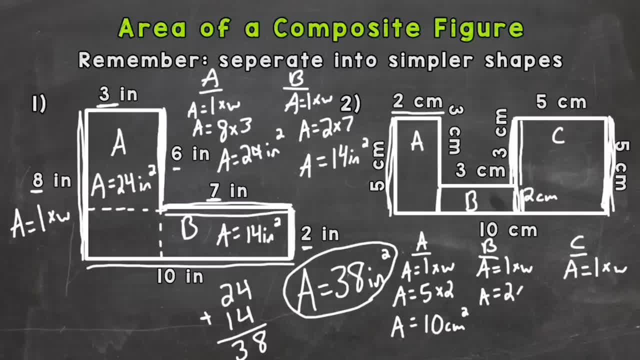 So our length is going to be 2 times the width of 3 centimeters, which is given. So 2 times 3 gives us 6 square centimeters. And lastly, for C, we have a square here, 5 by 5 square. 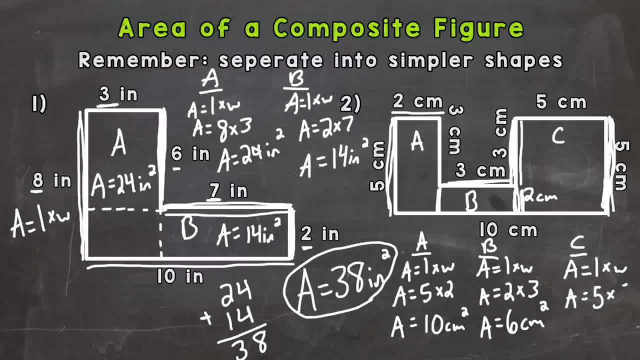 So our length is 5, and our width is 5.. So our area is going to be 25 square centimeters. So now we need to add these together: 10 plus 6 plus 25.. 10 plus 6 is 16, plus 25 is going to give us 41.. 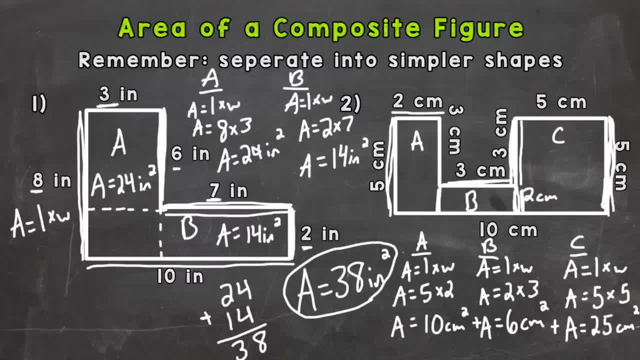 So the area I'm going to put it in the top right corner, where I have some room Area, equals 41 square centimeters, And that's our final answer for number 2.. Now, just like number 1, there's multiple ways to solve for that answer. 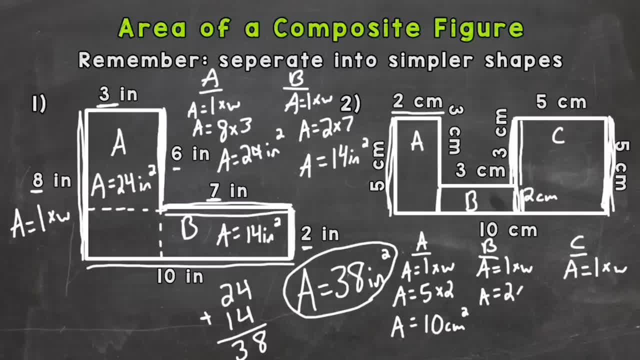 So our length is going to be 2 times the width of 3 centimeters, which is given. So 2 times 3 gives us 6 square centimeters. And lastly, for C, we have a square here, 5 by 5 square.